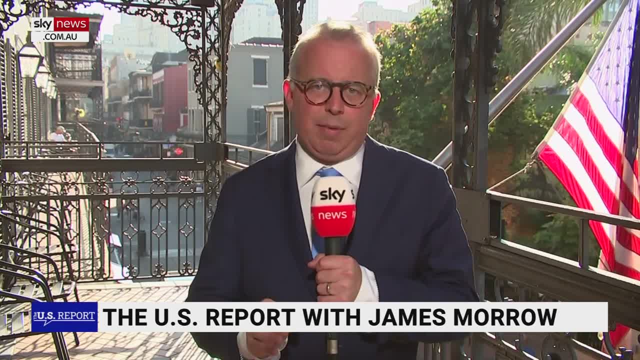 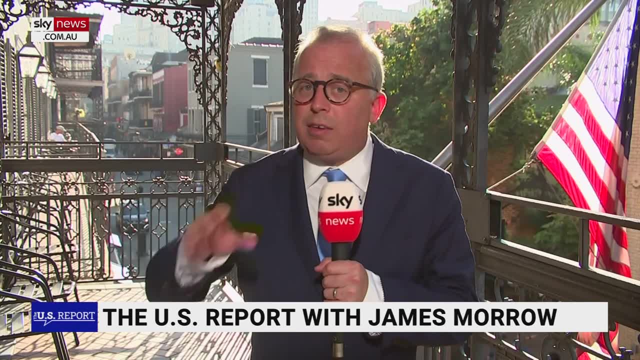 One of the things that this is leading to is an enthusiasm gap. Republicans look far keener than Democrats to vote heading into the midterms this time around, which means in a country that, unlike Australia, does not have compulsory voting, the Republicans also have the edge. 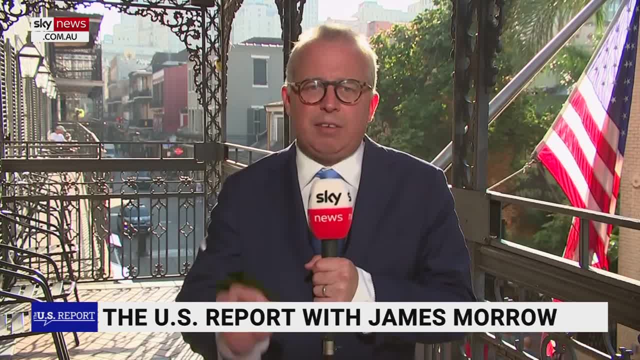 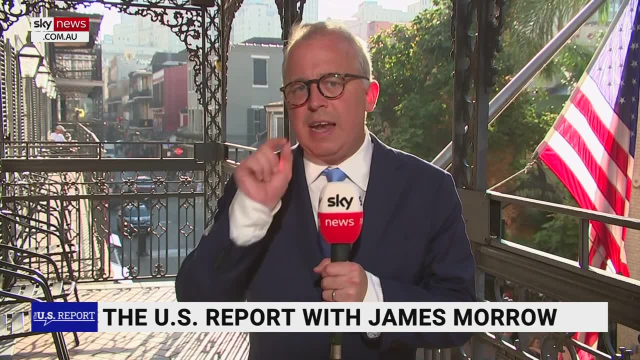 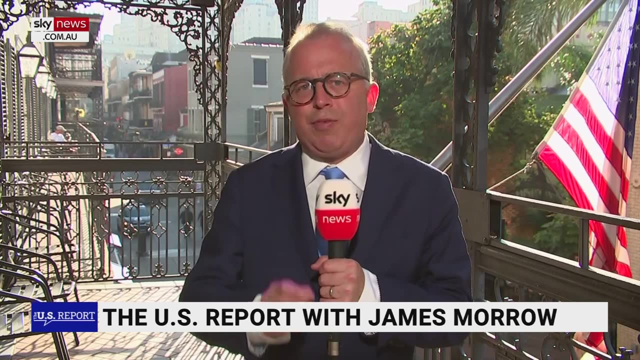 This is especially the case in Florida, where Governor Ron DeSantis has put himself in the box seat for a 2024 or 28 presidential run precisely because he listened to voters and not the elites, on everything from COVID to the economy. Earlier this week, I spoke with Florida State University Professor Lana Atkinson. 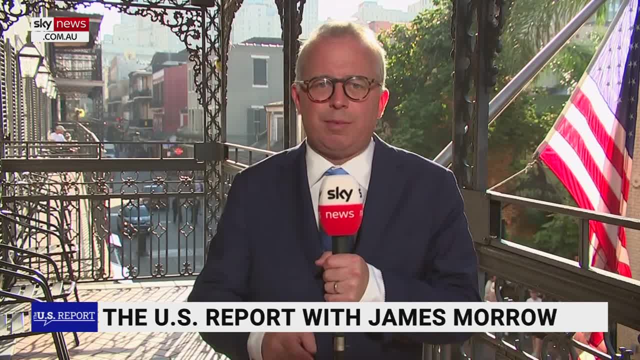 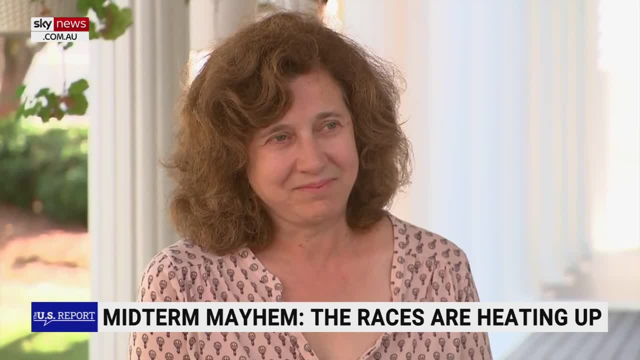 an elections expert who explained what this means in the Florida race. Lana Atkinson, thank you so much for joining us on the US Report. Tell me you're here in Florida. You're an elections expert Here in Florida. what are we seeing going into next Tuesday? 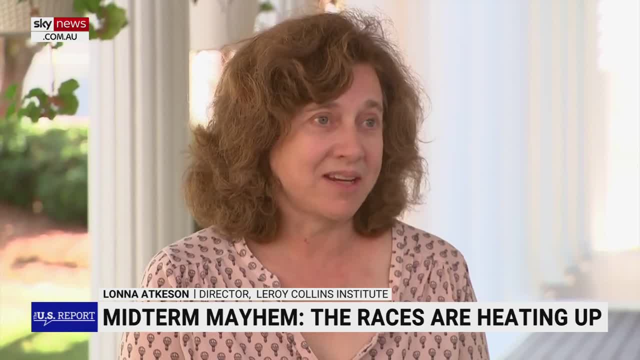 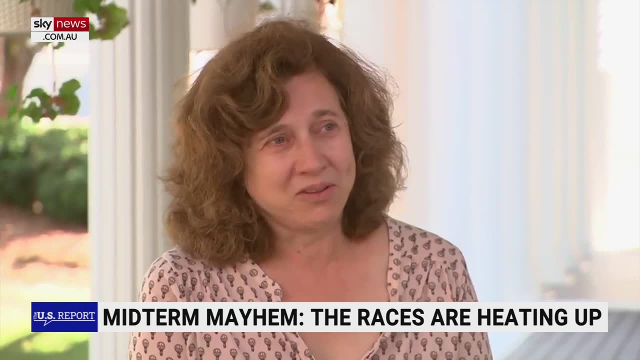 Well, we're seeing here in Florida a lot of activity for early voting and vote-by-mail. In fact, for the first time ever we have seen Republican turnout being seen in the state of Florida. It's going to be higher than Democratic turnout in the early voting period. 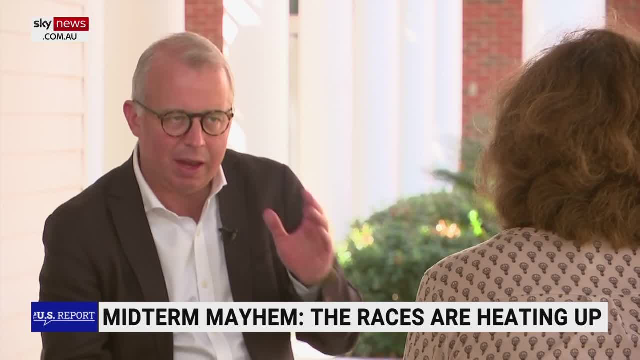 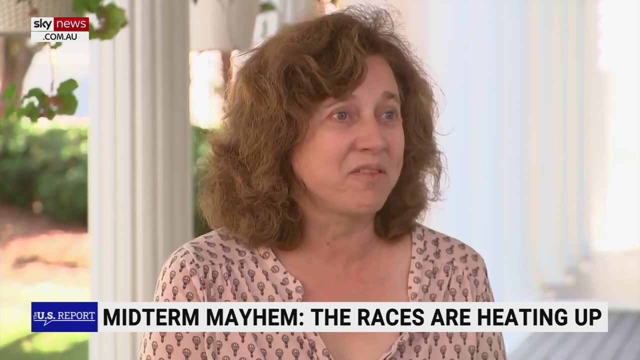 Right now Ron DeSantis and Marco Rubio. they're ahead in the polls here. They're ahead in the early voting. Are you seeing this carrying through statewide and a Republican trend nationally? Well, if we assume that all of the ballots who voted Republican are for Republicans. 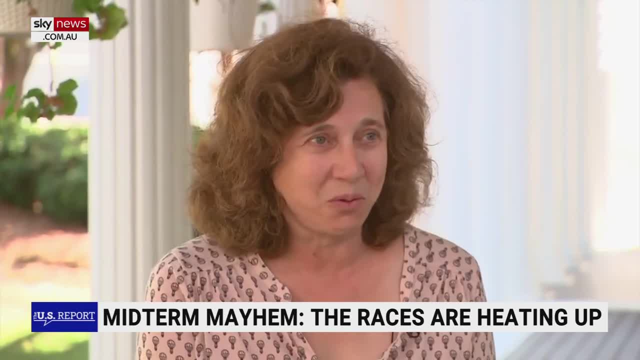 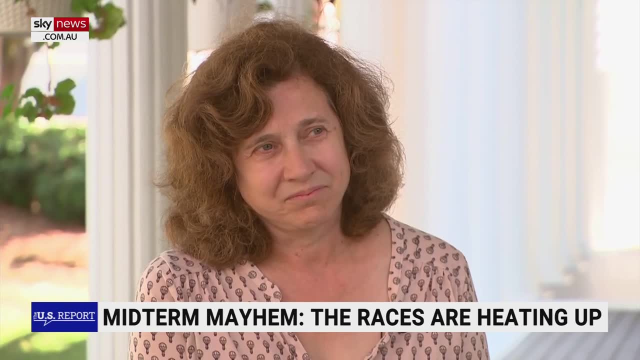 that would be the case, But of course we don't know what those ballots hold within them. What's driving the run to the Republican Party in Florida? Is it the lack of opposition? Is it Ron DeSantis' national profile that's building? 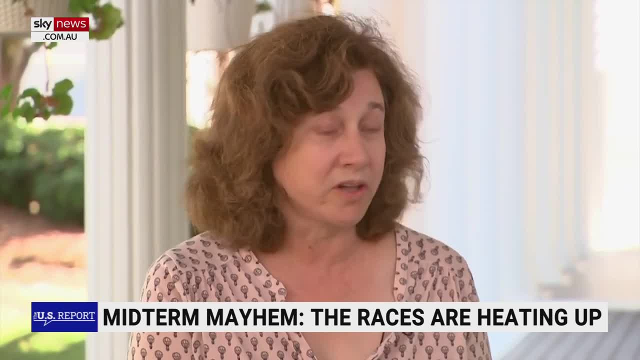 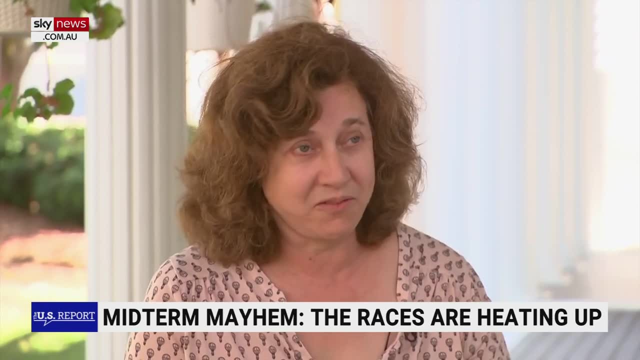 Or is it some other X-Factor? Well, I think these are sort of long-term trends going on in the South In particular. if we look at a long-term chart of Florida, we see that Democratic Party identification has been declining over time. 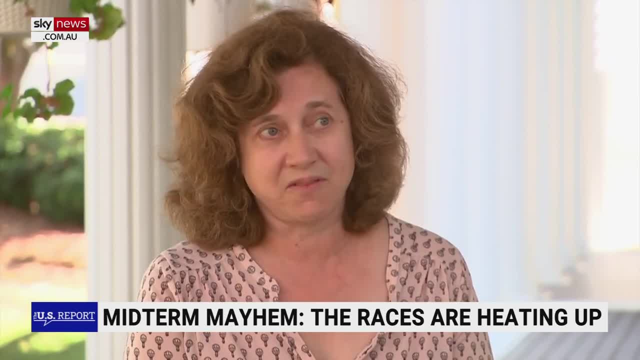 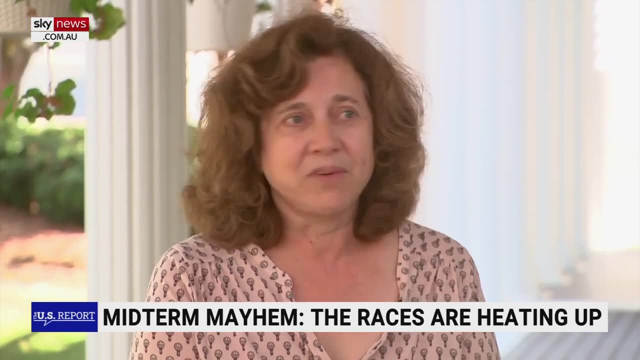 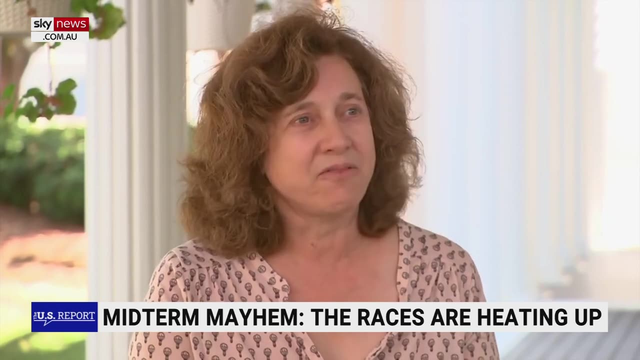 I think that in the last couple of years we've seen a huge influx of sort of immigrants from other states who are attracted to Florida for various reasons, perhaps policies that came in under COVID and things like that. So there's been sort of a lot of forces at play. 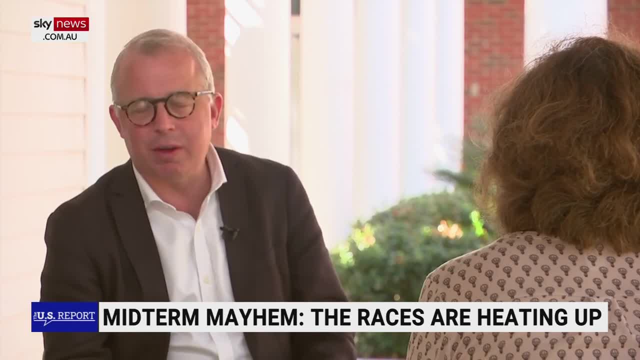 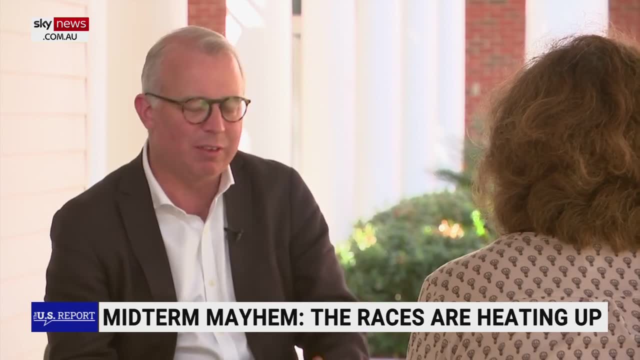 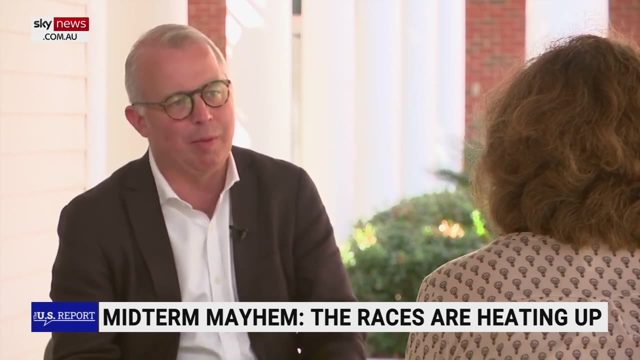 And I think that's going to play to lead us down this road. There's concern among some in Florida and Texas that all these blue state voters who are coming in are going to import the failed policies of Democratic states. Is that happening, Or are they really here because they are committed to more conservative, Republican red state policies?